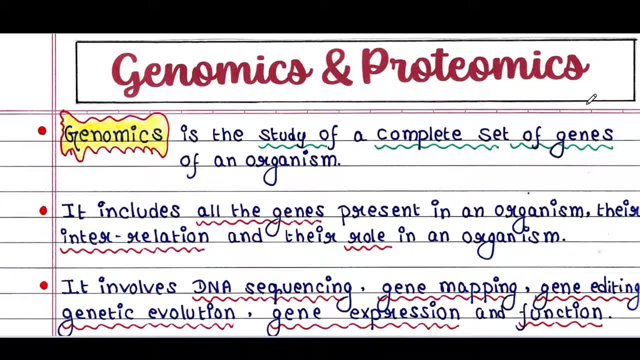 Hey guys, this is Malinki. Welcome back to my channel, Voice of Malinki. Today we will talk about genomics and proteomics And if you are new in my channel, please subscribe my channel. And if you like my video, please do like, comment and share my video. 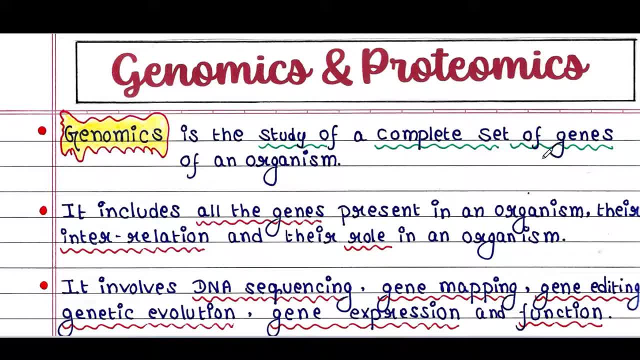 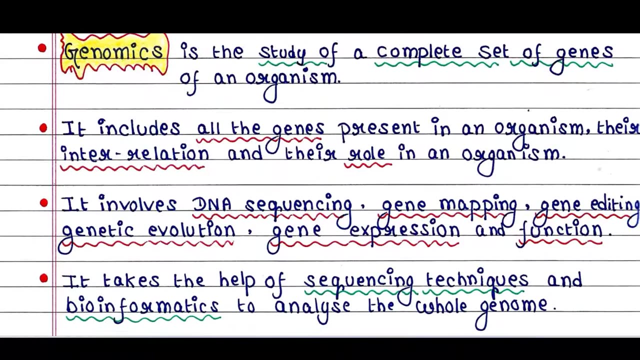 So genomics is the study of a complete set of genes of an organism, So it considers all the genes of an organism. It includes all the genes present in an organism, their interrelation and their role in an organism. It involves DNA sequencing, gene mapping, gene editing. 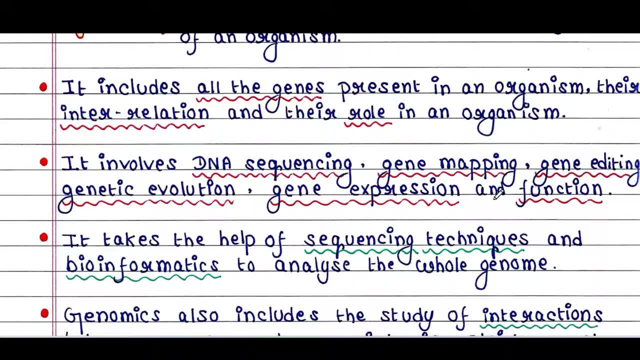 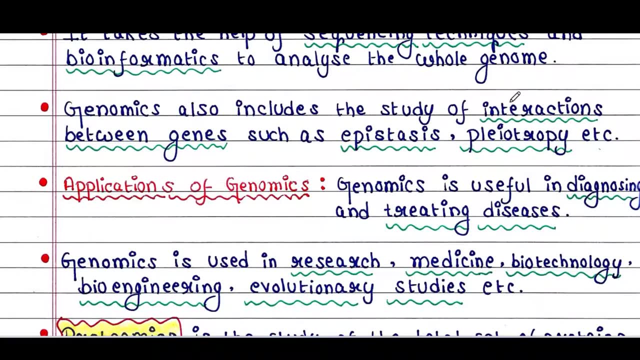 genetic evolution, gene expression and function. It takes the help of sequencing techniques and bioinformatics To analyze the whole genome. Genomics also includes the study of interactions between genes such as epistasis and pleiotropy. Let's talk about some applications of genomics. 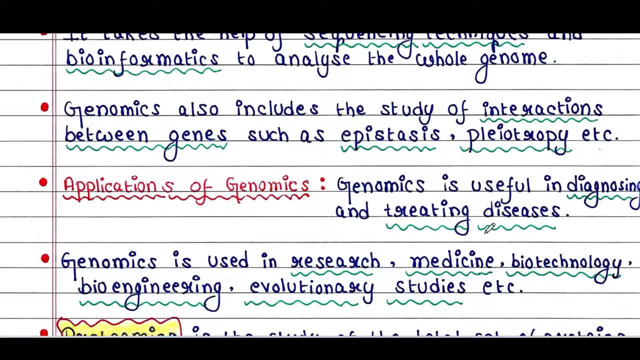 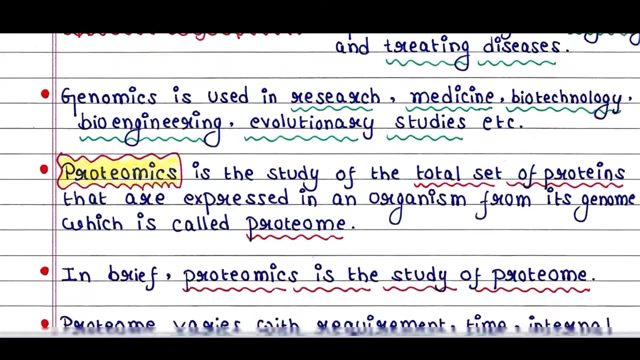 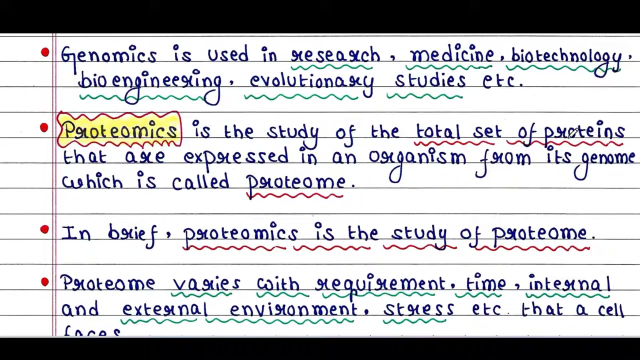 Genomics is useful in diagnosing and treating diseases. So using genomics, we can compare the genome of a healthy and a diseased individual. Genomics is used in research, medicine, biotechnology, bioengineering, evolutionary studies, etc. Let's talk about proteomics now. So proteomics is the study of the total set of proteins. 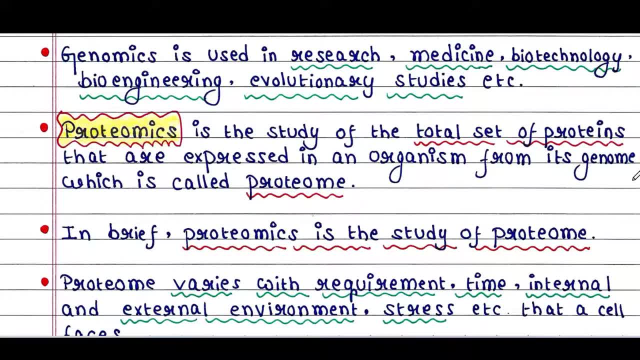 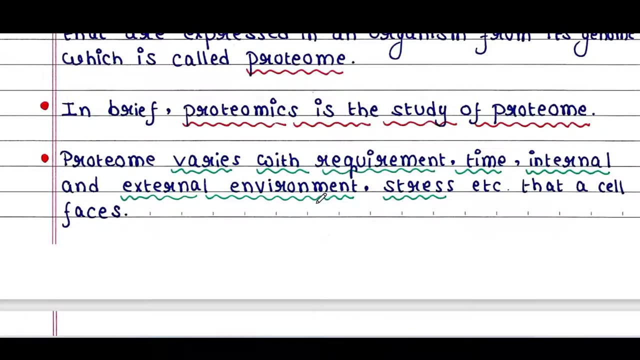 that are expressed in an organism from its genome, which is called proteome. In brief, proteomics is the study of proteomes. Proteome varies with requirement, time, internal and external environment, stress, etc. that a cell faces, Since different cells express different proteins right And it depends on these factors. 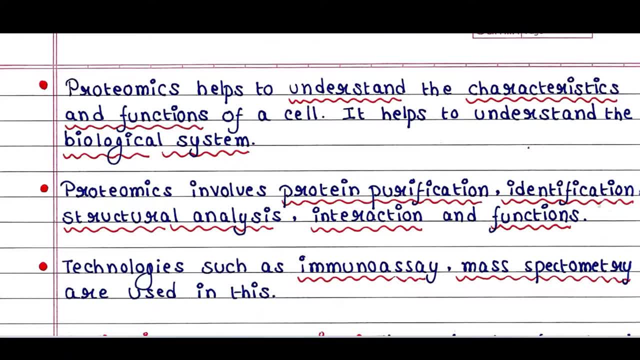 Proteomics helps to understand the characteristics and functions of a cell. It helps to understand the function of a cell. It helps to understand the characteristics and functions of a cell. It helps to understand the function of a cell And it helps to understand the biological system, Since proteins control the function of a cell. ultimately, 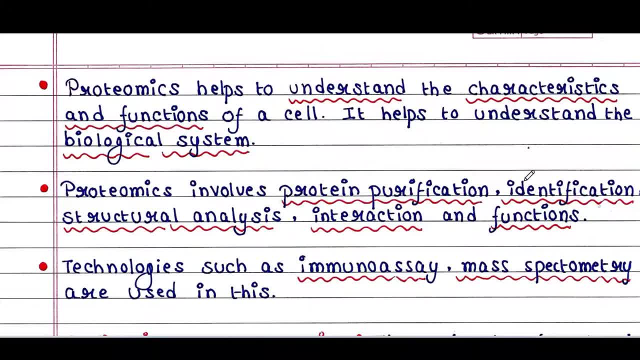 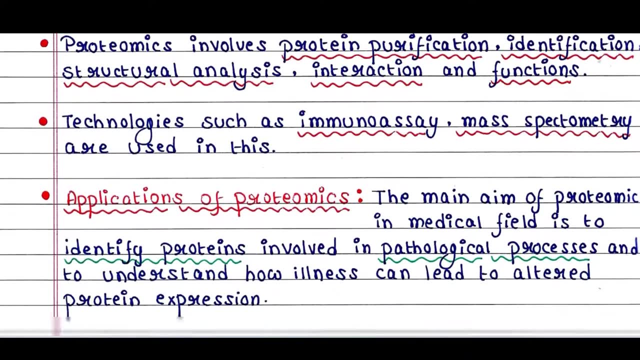 Proteomics involves protein purification, identification, structural analysis, interaction and function. Technologies such as immunoassay mass spectrometry are used in these. Let's talk about some applications of proteomics. Let's talk about some applications of proteomics. 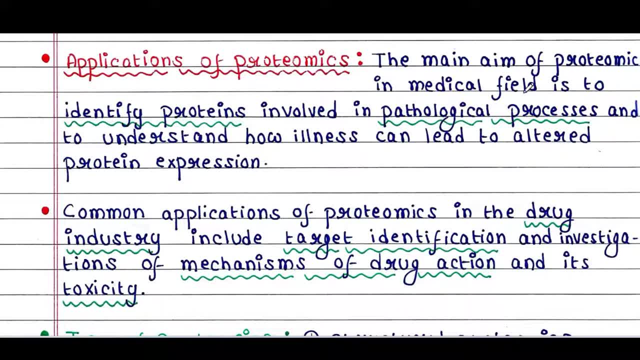